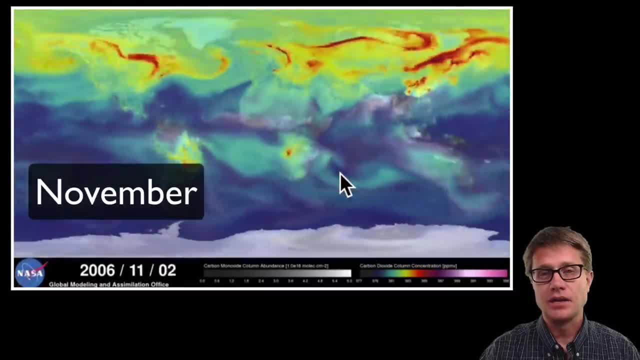 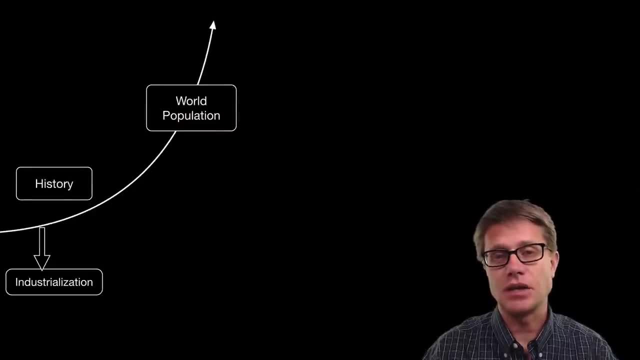 the leaves start to fall, That carbon dioxide comes back again, And so it's not equal impact to the environment. And so we've learned so far that with industrialization, you see exponential growth in a population And so the population increases in. that is impacting the environment. 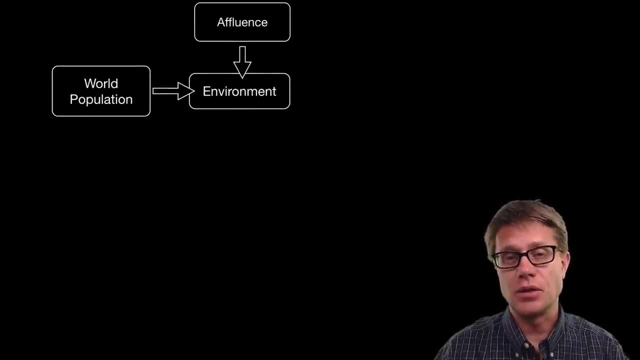 But it's not only the number of people, It's the number of people, It's the number of people, people, It's the affluence of those people, It's how much they're consuming, And it's also their technology. Now, some technology can actually help the environment, And so 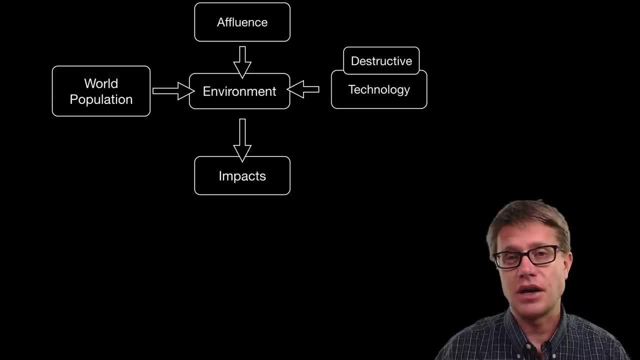 I'm talking about destructive technology. It's impacting the environment. One way to measure that is using the iPad equation. You don't actually have to calculate it, But it's combining these three things: The population, the affluence and the destructive technology. 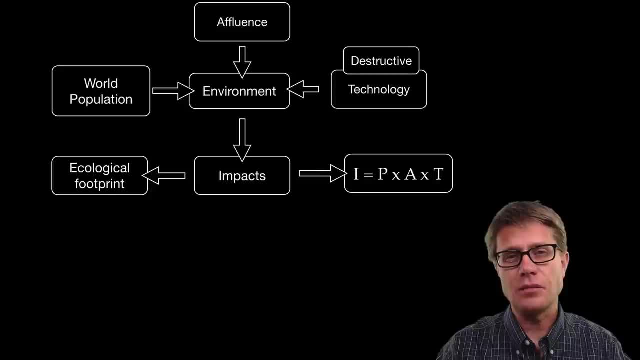 An analogous model is the ecological footprint. It measures how much of the earth do we need to support that industry. Now, these are feedback loops, And so all of these are going to put impacts on the population itself. Another big one, aside from population, is the economy. 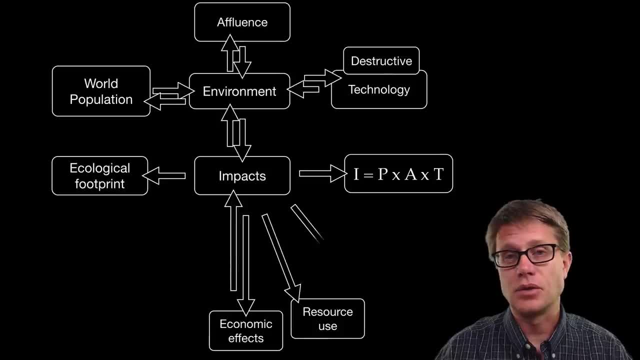 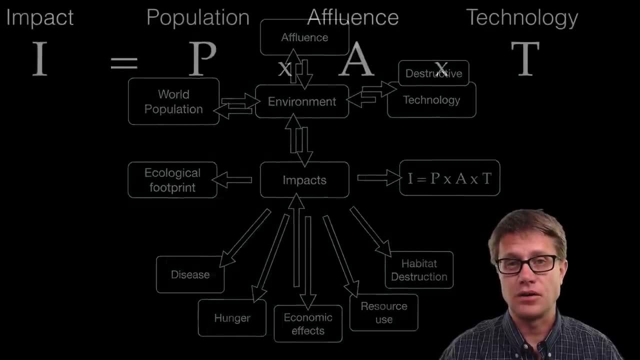 If the economy grows too much, that is going to consume resources and destroy habitat, But if the economy is not big enough in certain countries, it can lead to disease and hunger, And so the iPad equation looks like this. It's pretty easy. On the left side we have 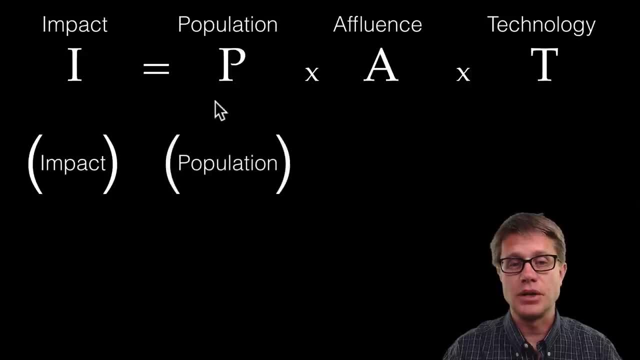 the impact. We then have the population. So in other words, the bigger the population, the larger the impact. If we are looking at affluence, that is going to be consumption per person. So if you have a house and several TVs and many cars, you are probably going to 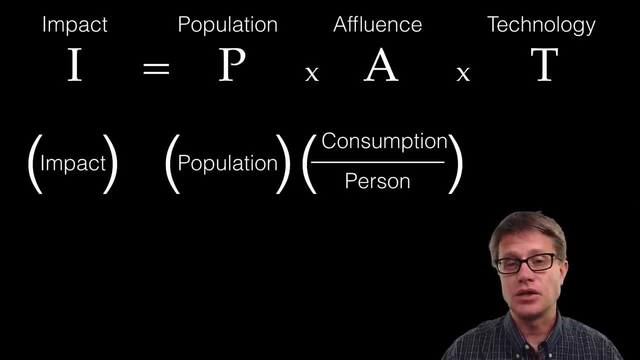 have more affluence than somebody who lives in a village in Africa. And then is that consumption actually harming the environment or impacting it? Well, it depends on what technology that is. And so let's give you an example. So let's look at a country. So this is Burundi. It's 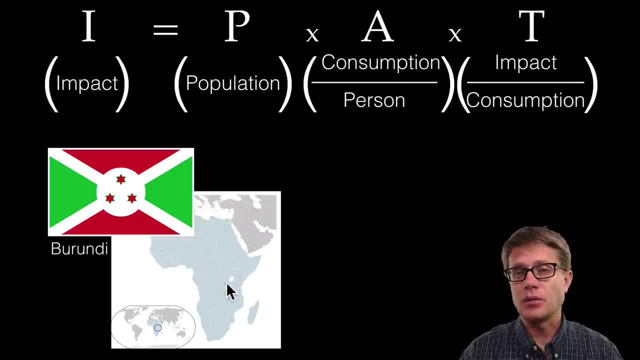 in the Rift Valley of Africa And they have a huge population And they have a huge population And so if we look at their population, there are about 9 million people that live there. So there is going to be a certain impact. If we look at how much money they make, the 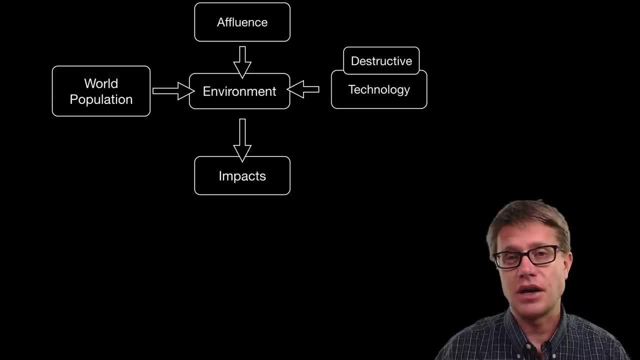 I'm talking about destructive technology. It's impacting the environment. One way to measure that is using the iPad equation. You don't actually have to calculate it, But it's combining these three things: The population, the affluence and the destructive technology. 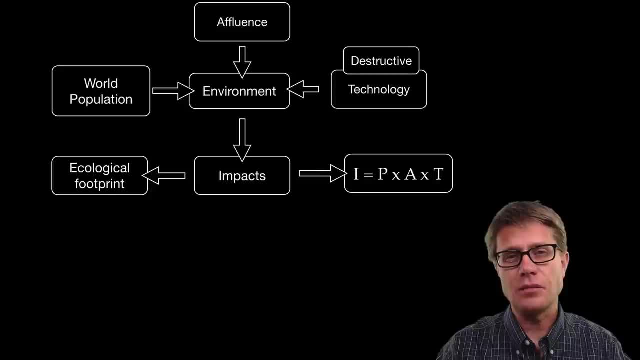 An analogous model is the ecological footprint. It measures how much of the earth do we need to support that industry. Now, these are feedback loops, And so all of these are going to put impacts on the population itself. Another big one, aside from population, is the economy. 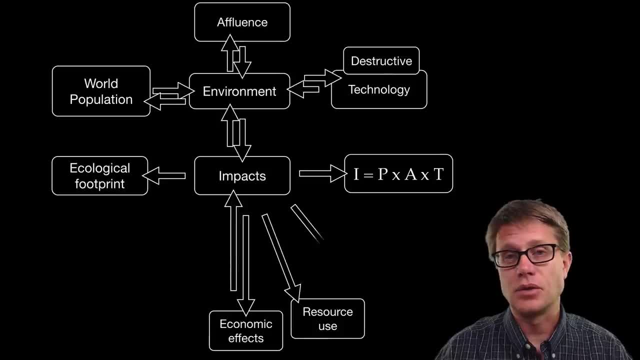 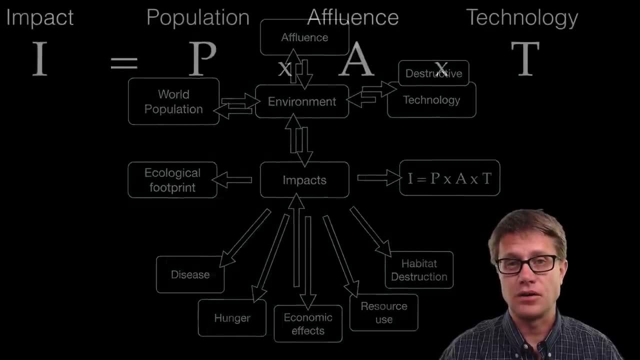 If the economy grows too much, that is going to consume resources and destroy habitat, But if the economy is not big enough in certain countries, it can lead to disease and hunger, And so the iPad equation looks like this. It's pretty easy. On the left side we have 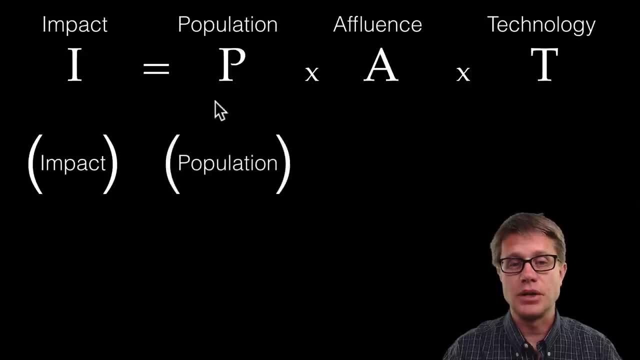 the impact. We then have the population. So in other words, the bigger the population, the larger the impact. If we're looking at affluence, that's going to be consumption per person. So if you have a house and several TVs and many cars, you're probably going to. 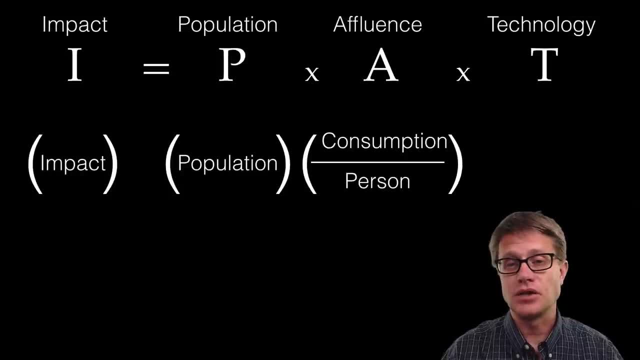 have more affluence than somebody who lives in a village in Africa. And then is that consumption actually harming the environment or impacting it? Well, it depends on what technology that is. And so let's give you an example. So let's look at a country. So this is Burundi. It's 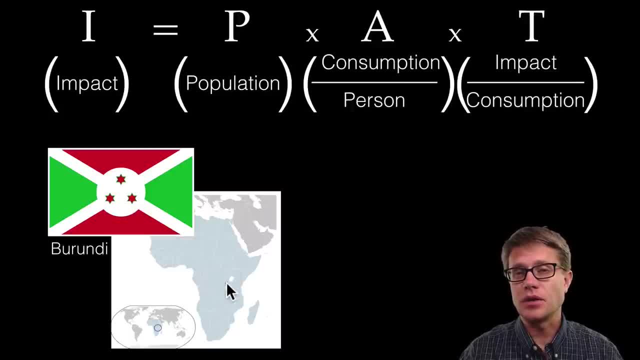 in the Rift Valley of Africa And it's a very large country And it's a very large population And so if we look at their population, there are about 9 million people that live there, So there's going to be a certain impact. If we look at how much money they make- the average- 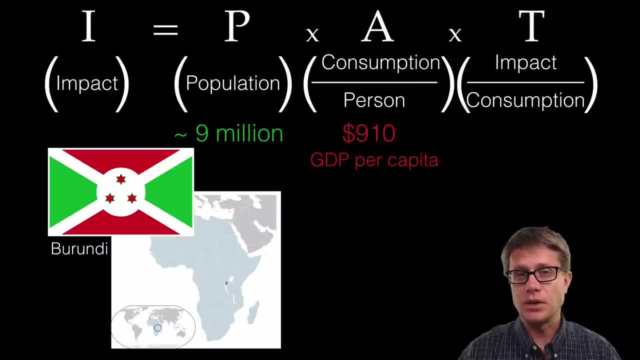 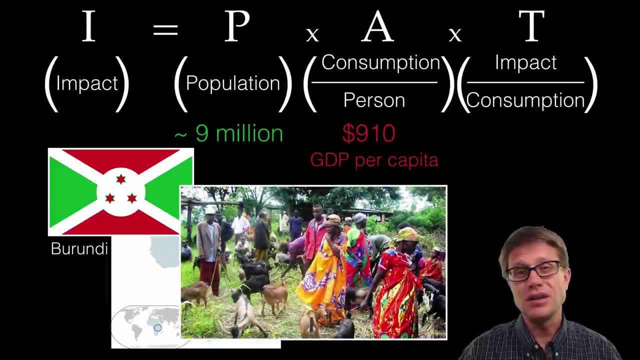 person makes $910 per year. What does that mean? They don't get much money, so there can't be much consumption. If we were to look at the major industry, it's going to be agriculture. Meat is rare because it's going to be highly expensive. If we look at transportation- bicycles- 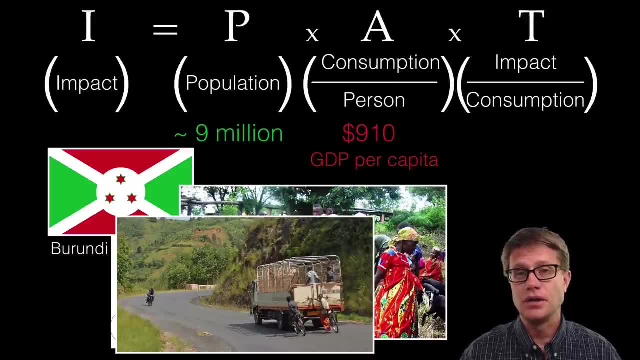 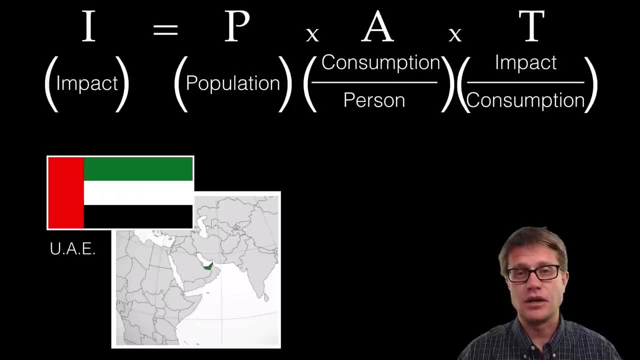 are really common. There's going to be a huge impact in Burundi on the environment. No, It's going to be relatively low. But if we look at another country- so this is the UAE or the United Arab Emirates- their population is 9 million as well. If we start to look at their consumption, however, 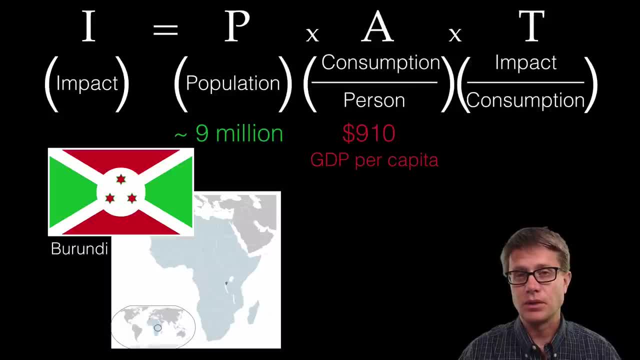 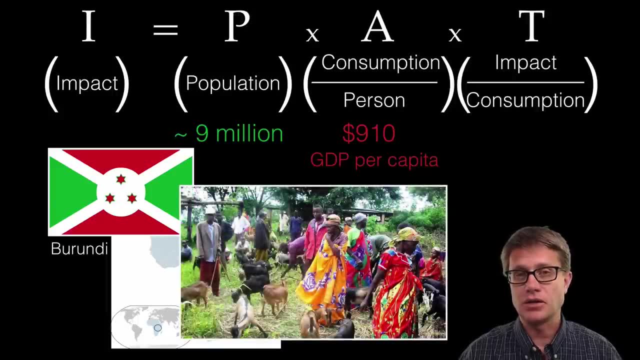 average person makes $910 per year. What does that mean? They don't get much money, so there can't be much consumption. If we were to look at the major industry, it is going to be agriculture. Meat is rare because it is going to be highly expensive. If we look at transportation- bicycles- 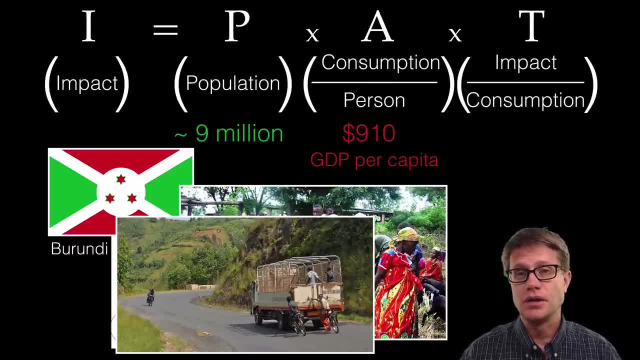 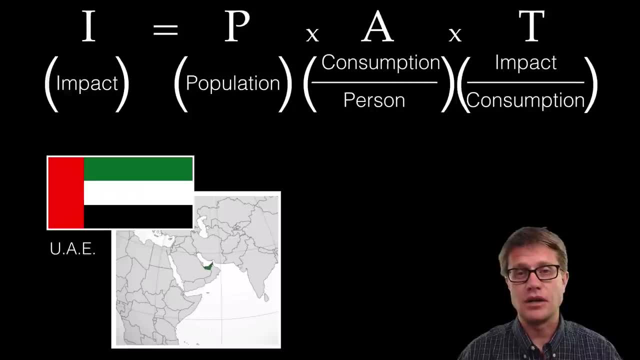 are really common. If we were to look at the food industry, we would see that there is a huge impact in Burundi on the environment. No, It is going to be relatively low. But if we look at another country- so this is the UAE or the United Arab Emirates- their population is 9 million. 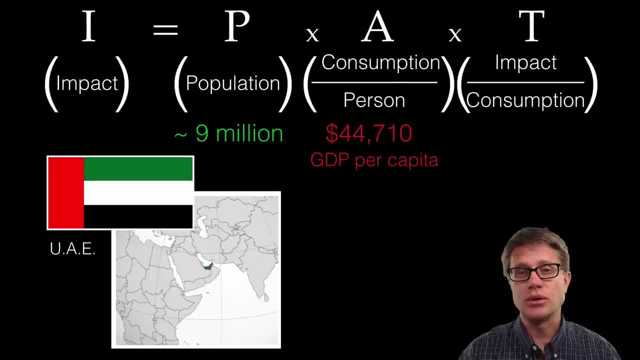 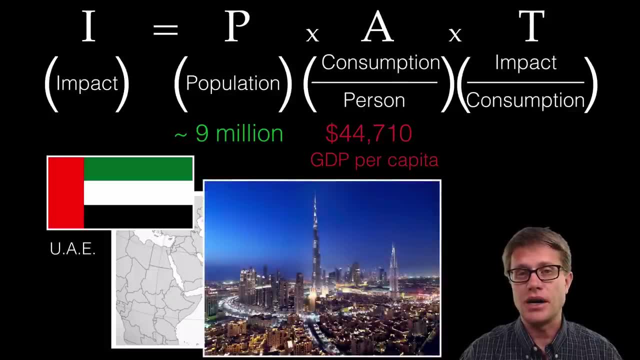 as well. If we start to look at their consumption, however, the average person there makes 50 times what somebody in Burundi makes. What does that mean? There is a lot more consumption per person. If we look at their technology- this is Dubai- you can see there is way more. 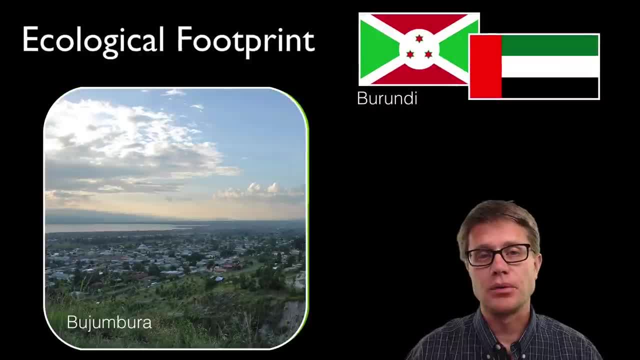 food, there is going to be a greater impact on the environment. If we look at Burundi- this is the capital of Burundi- You can see there is not a lot of industry, And so that means it is going to have a really small footprint. It does not consume much of the Earth's area. 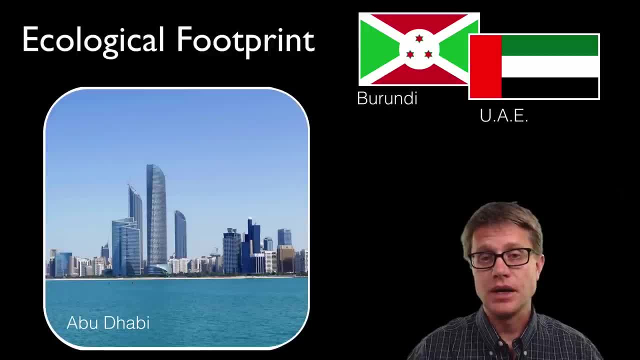 If we look at something like UAE, there is way more industry, And so if we were to put values to this, the ecological footprint of Burundi is going to be less than 1 global hectare per person. It is going to be relatively small If we look at it what it is in the 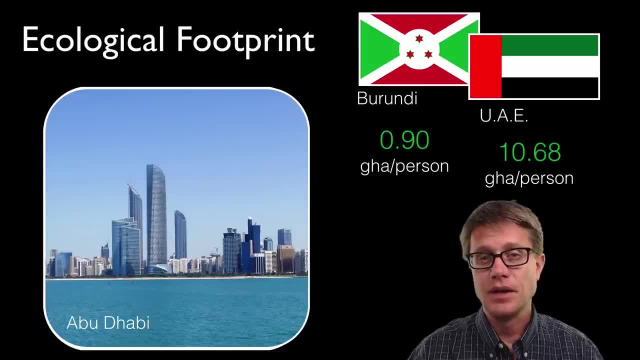 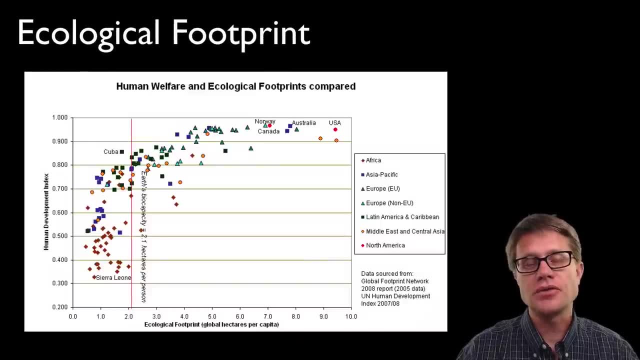 is in the UAE, it is going to be about 12 times that. That means it is going to have a larger ecological footprint. It is going to consume more of the earth's resources. So this graph is kind of interesting. On the bottom we have the ecological footprint And on the right 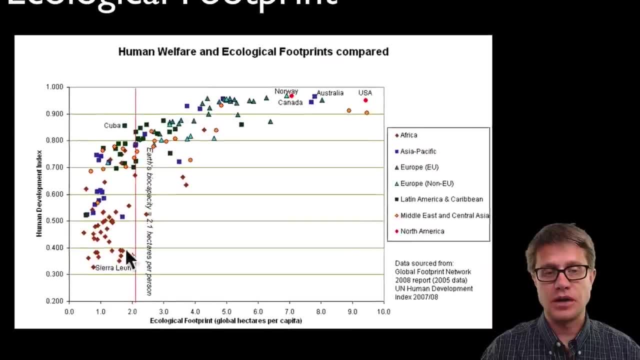 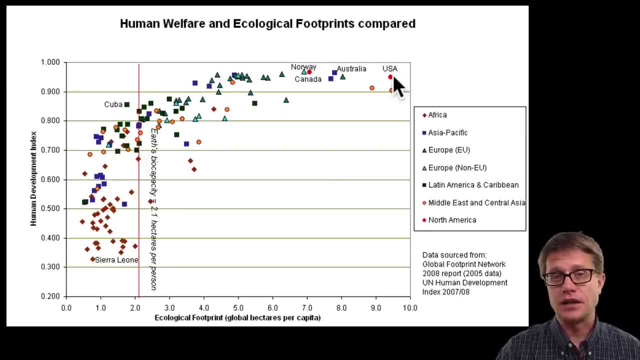 side. we have a development index And so these are going to be the developing countries and these are going to be the developed countries. So the US is going to have high development index, It is highly developed and it is also going to have a very large ecological footprint. 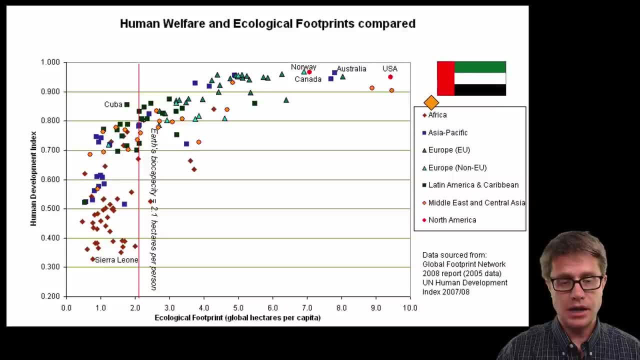 And so where do you think the UAE is going to be? It is going to be way out here. So it is going to have a high footprint and it is going to be highly developed. It has more impact on our planet. It has got a larger economy. If we were to say, where is Burundi? 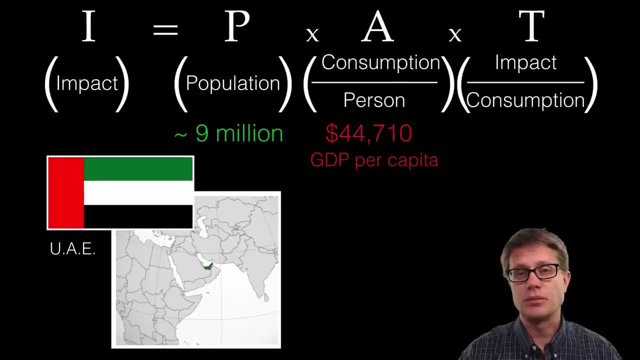 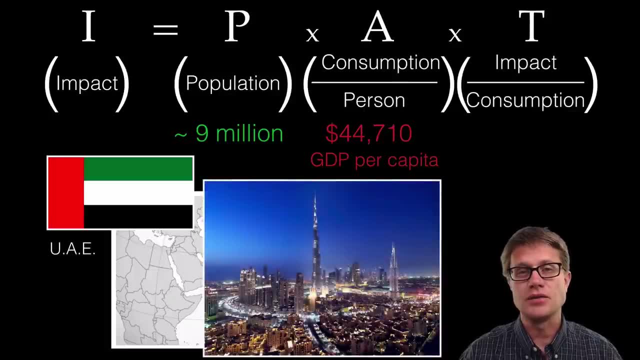 the average person there makes 50 times what somebody in Burundi makes. What does that mean? There's a lot more consumption per person. If we look at their technology- this is Dubai- you can see there's way more technology, Way more burning of fossil fuels. There's going. 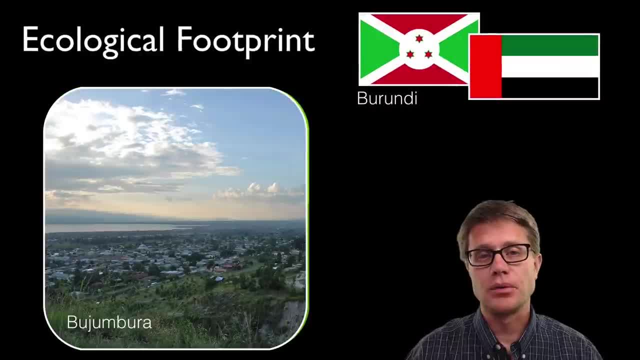 to be a greater impact on the environment. If we look at Burundi- this is the capital of Burundi- you can see there's not a lot of industry, And so that means it's going to have a really small footprint. It doesn't consume much of the earth's area. If we look 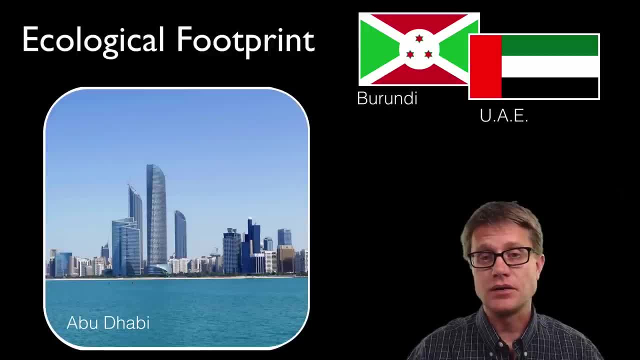 at something like UAE. there's way more industry, And so if we were to put values to this, the ecological footprint of Burundi is going to be less than 1 global hectare per person. It's going to be relatively small If we look at it what it is. 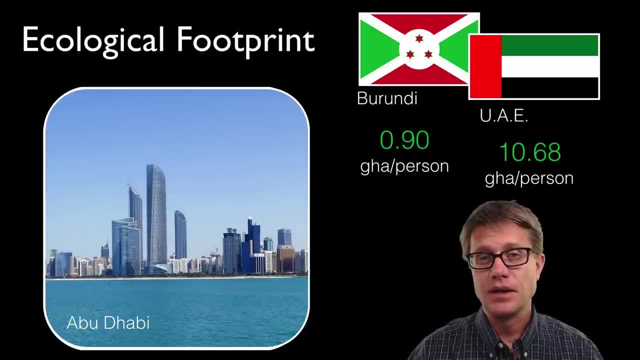 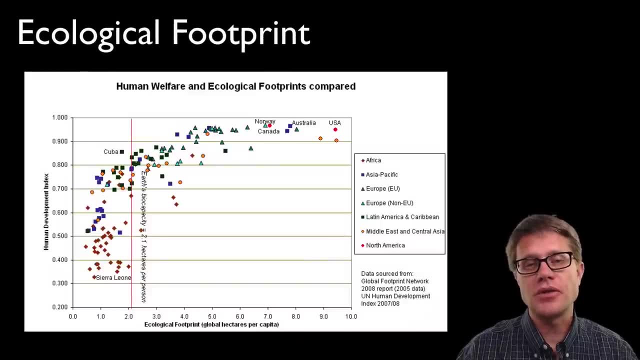 in the UAE it is going to be about 12 times that. That means it is going to have a larger ecological footprint. It is going to consume more of the earth's resources. So this graph is kind of interesting. On the bottom we have the ecological footprint And on the right 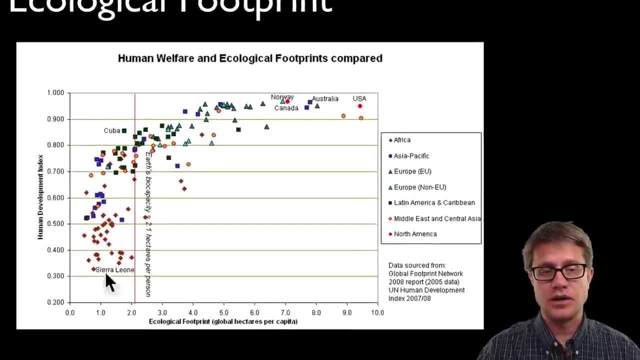 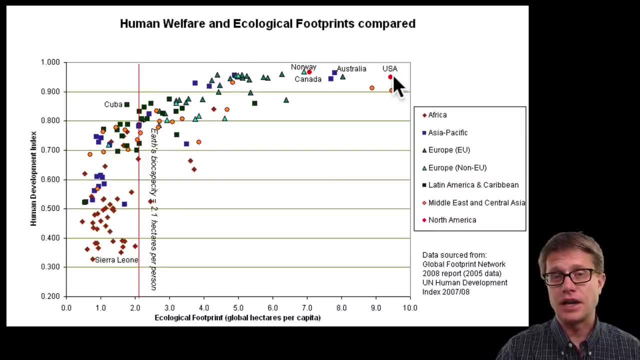 side. we have a development index And so these are going to be the developing countries and these are going to be the developed countries. So the US is going to have high development index, It is highly developed and it is also going to have a very large ecological footprint. 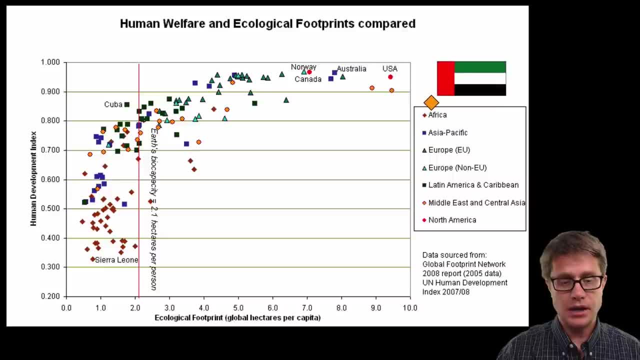 And so where do you think the UAE is going to be? It is going to be way out here. So it is going to have a high footprint and it is going to be highly developed. It has more impact on our planet. It has got a larger economy. If we were to say, where is Burundi? 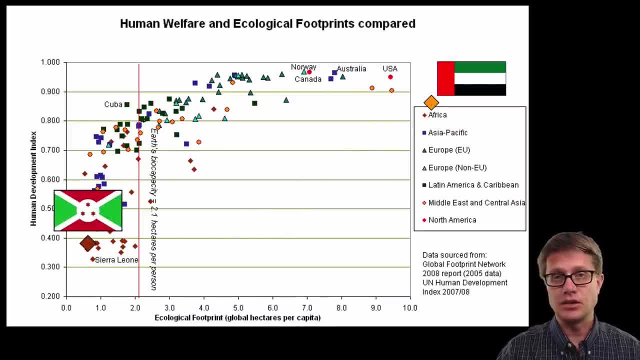 going to be. It is going to be way down here. It is a developing nation And so you can see the general trend is, as countries develop, they will move up and then they will move across, And that means they are going to start to have more of a 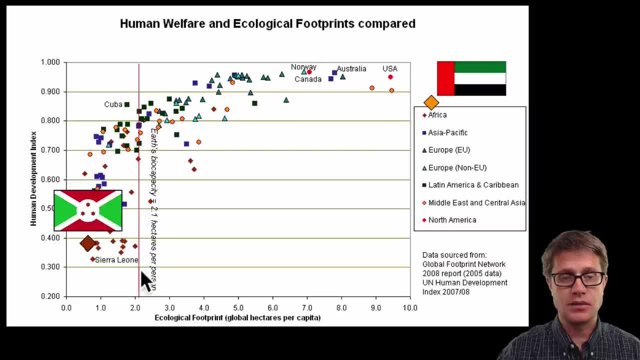 global impact on the planet. Now, this line is interesting. This line, right here at 2.1 global hectares per person, is the biocapacity, It is what our earth can support, And so you can see that a lot of countries are actually exceeding that. And so, going back to our model, 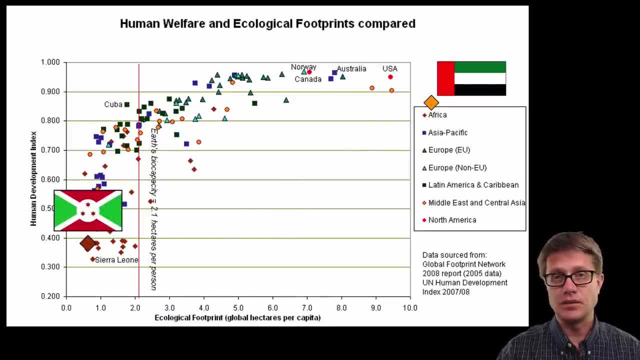 going to be. It is going to be way down here. It is a developing nation And so you can see the general trend is, as countries develop, they will move up and then they will move across, And that means they are going to start to have more of an 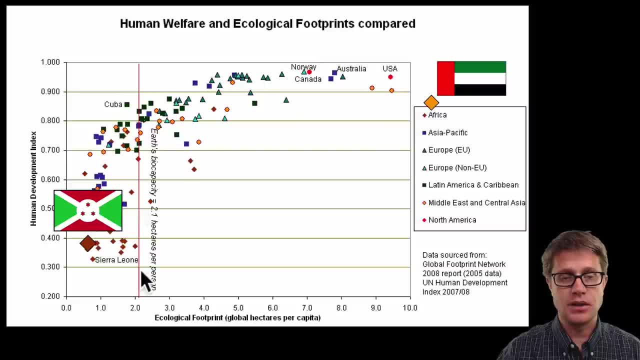 impact on the planet. Now, this line is interesting. This line right here, at 2.1 global hectares per person, is the biocapacity, It is what our earth can support, And so you can see that a lot of countries are actually exceeding that. And so, going back to our model again, 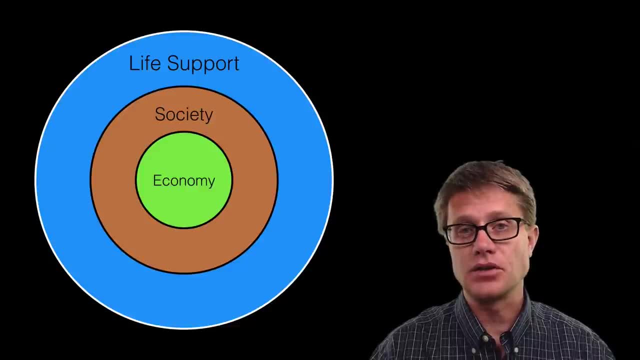 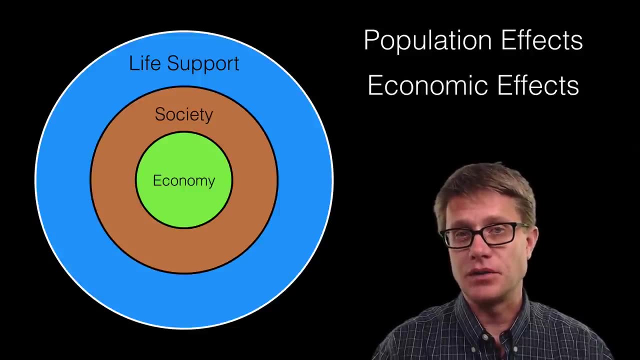 it is the society and the economy, And so as the population gets larger, we are going to have population effects on the environment. But the economy can affect it as well. If the economy is too large, then we have too much of an impact. But 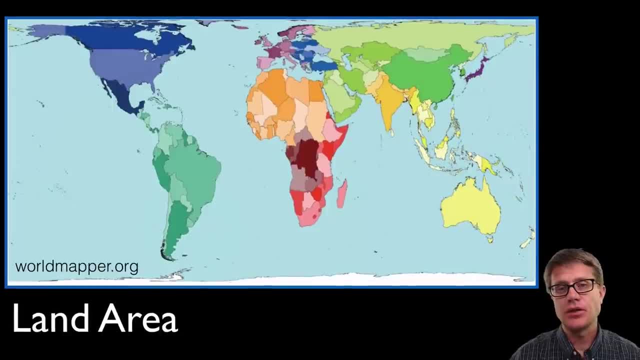 if it is too small, that can impact the society itself. To illustrate how the population and the economy can impact the environment and therefore the population, we are going to use worldmapperorg. It is a great website, And so let me show you what you can do. So this. 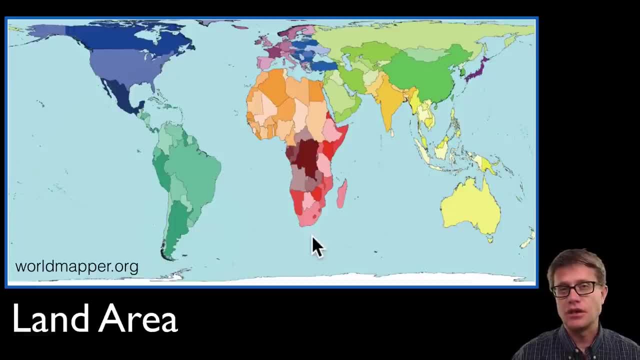 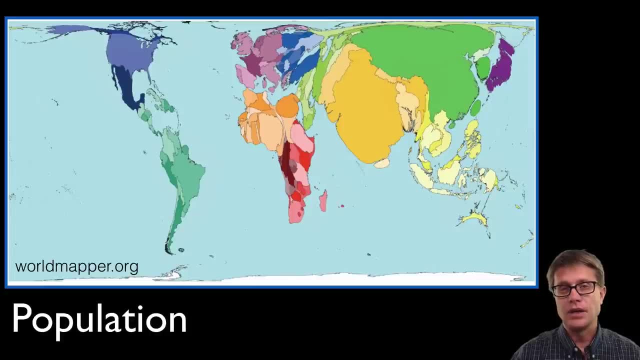 is a map of the world with all the countries. What you can do is you can change the size to represent another characteristic. So this is what the earth would look like if the countries represented the actual population. So you can see that some place like Canada shrinks. 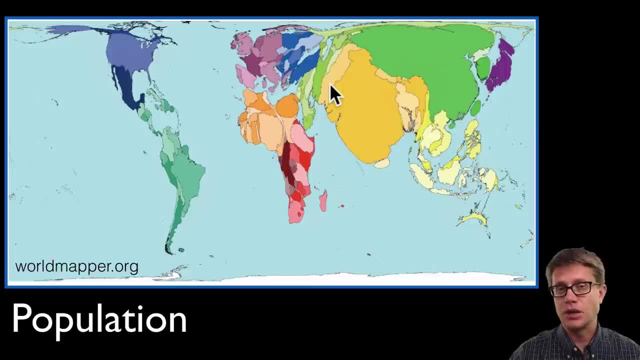 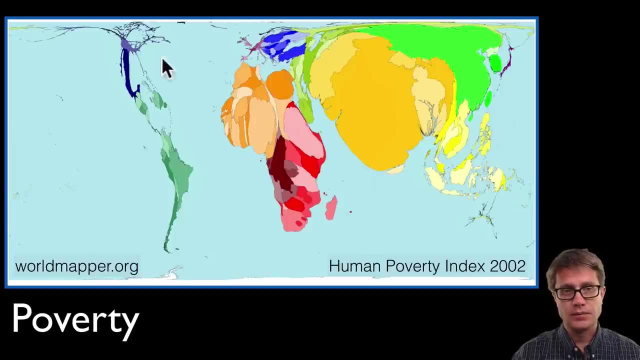 But China and India and Pakistan are going to get much larger And that is because they have a really high population. If we were to look at poverty, what happens? Well, America shrinks to almost nothing. Same with Western Europe, But we can see high poverty in India. 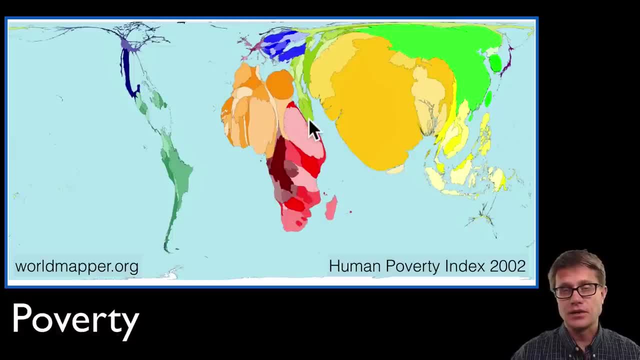 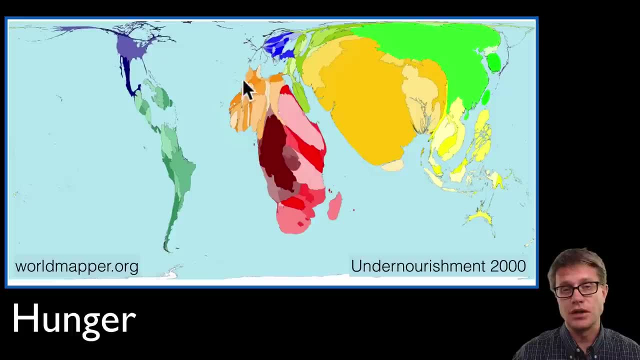 Some poverty in China And we have high poverty in Africa, And so this is going to impact the people. And so, if we look at hunger, for example, we are going to have high undernourishment in Africa and we are going to have high undernourishment in India. It has that double hit of a high population and high 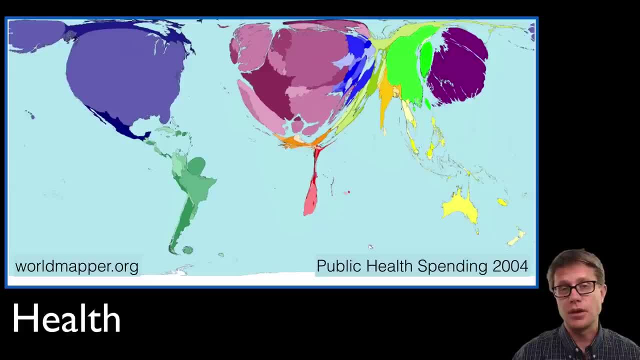 poverty. We could also look at health, And so this is health public spending And you can see it is going to be much greater in America and in Japan and in Western Europe. Well, how does that impact disease? for example, This is going to be the HIV prevalence You. 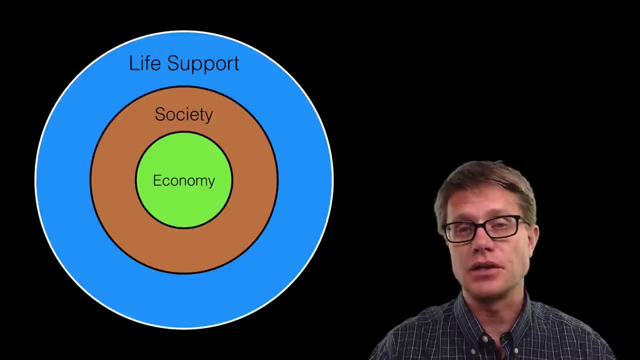 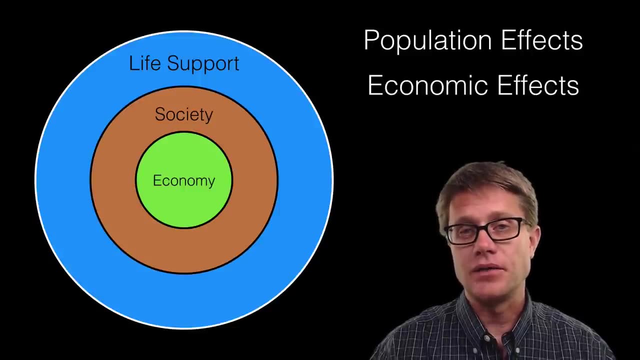 again, it is the society and the economy, And so as the population gets larger, we are going to have population effects on the environment, But the economy can affect it as well. If the economy is too large, then we have too much of an impact, But if the economy is too, 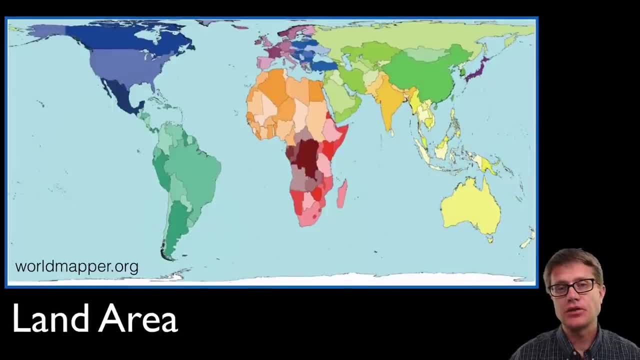 small, then that can impact the society itself. To illustrate how the population and the economy can impact the environment and therefore the population, we are going to use worldmapperorg. It is a great website, And so let me show you what you can do. So this is a map of the 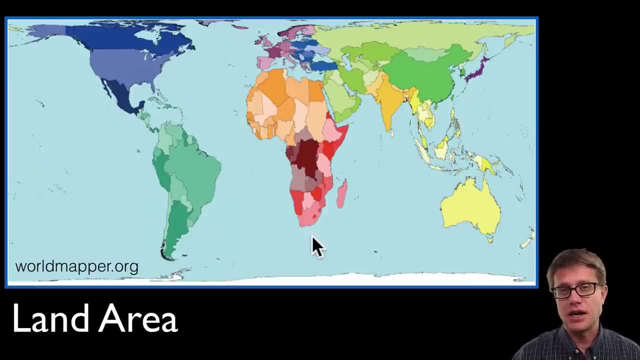 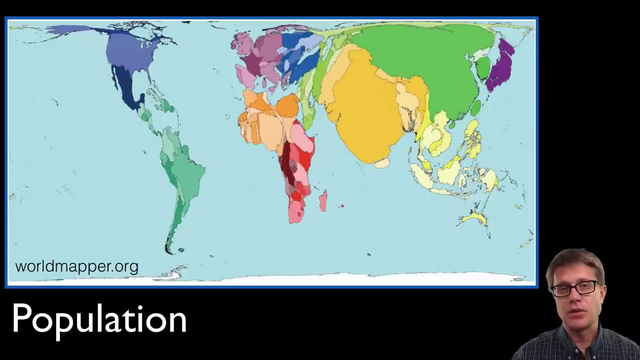 world with all the countries. What you can do is you can change the size to represent another characteristic. So this is what the earth would look like if the countries represented the actual population. So you can see that some place like Canada shrinks And then you 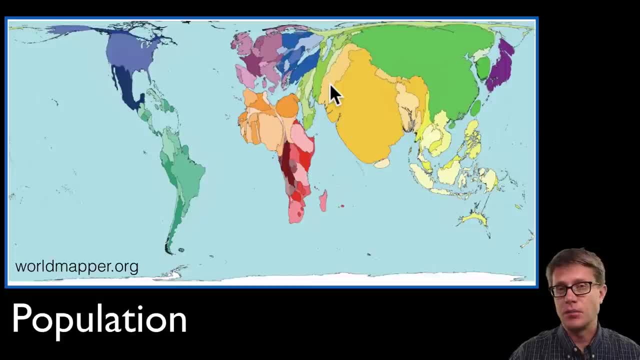 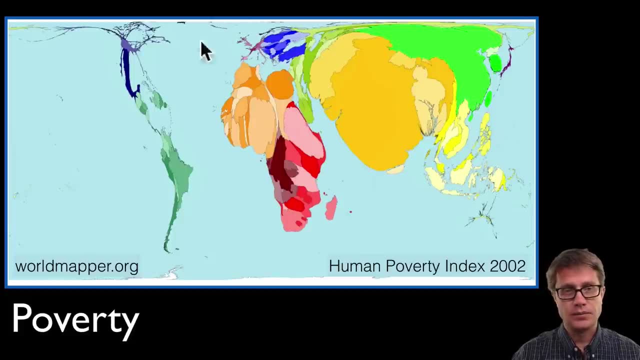 can see that some states like Spain and India are going to have higher poverty, But China and India and Pakistan are going to get much larger And that is because they have a really high population. If we were to look at poverty, watch what happens- Well, America shrinks to. 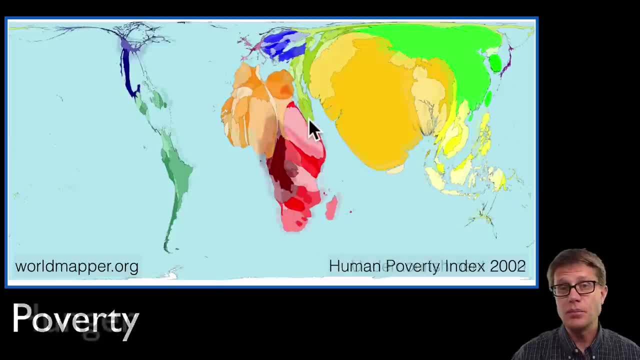 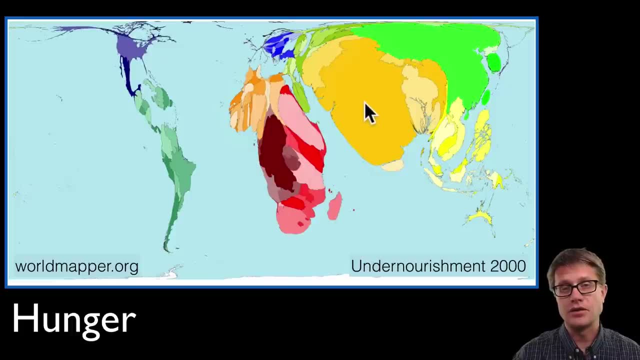 almost nothing Same with western Europe, But we can see high poverty in India, Some poverty in China And we have high poverty in Africa, And so this is going to impact high undernourishment in India. It has that double hit of a high population and high poverty. 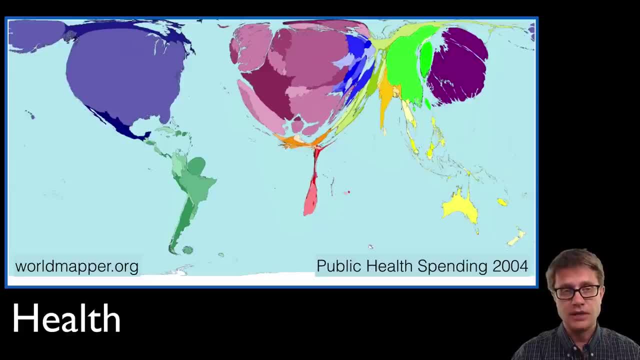 We could also look at health, And so this is health public spending And you can see it is going to be much greater in America and in Japan and in Western Europe. Well, how does that impact disease? for example, This is going to be the HIV prevalence You can. 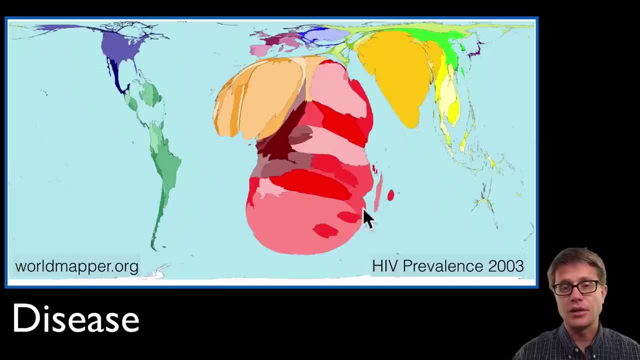 see it is going to be low in areas like Japan, But incredibly high where we are not spending much money on public health, So incredibly high. in certain areas of Africa It is 2 and sometimes 3 out of 10 adults are going to have HIV. If we look at income, we see that. 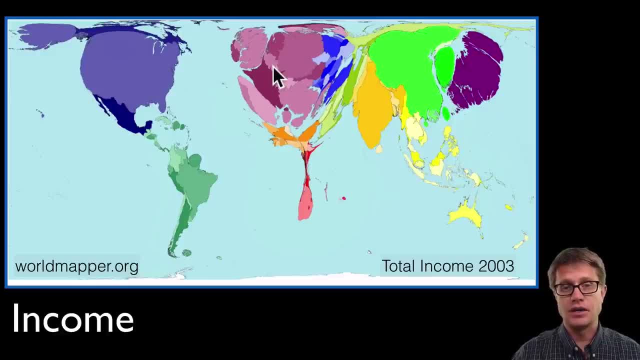 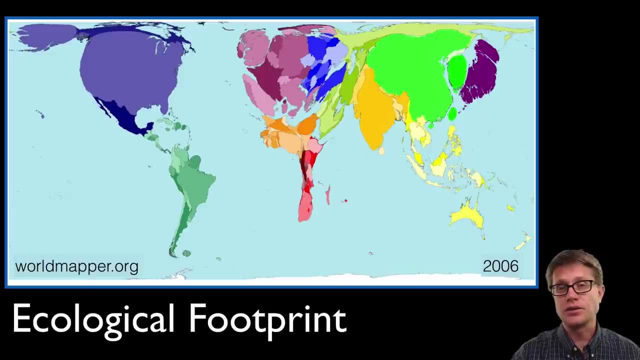 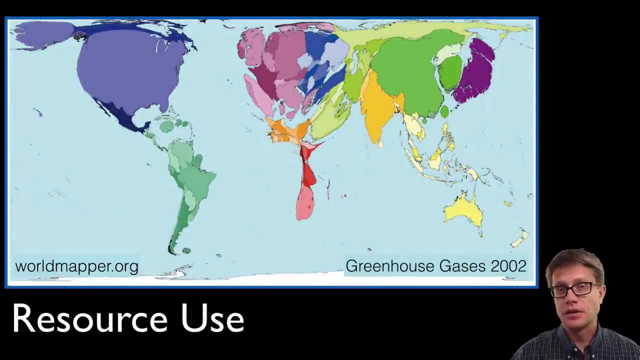 inverse relationship where we are going to see the developed nations having a higher income, Especially like Western Europe and the United States. How does that impact ecological footprint? It is going to be almost a direct relationship there. The greater the economy is, it is putting more impacts on the earth.